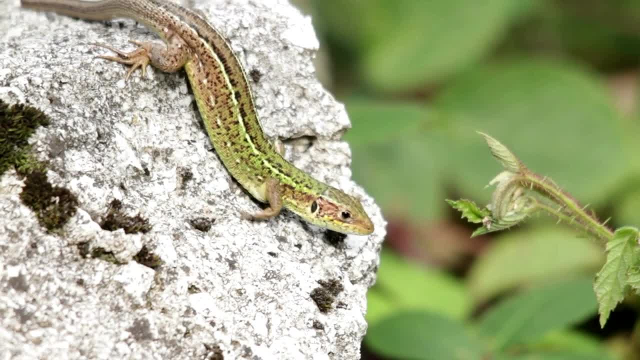 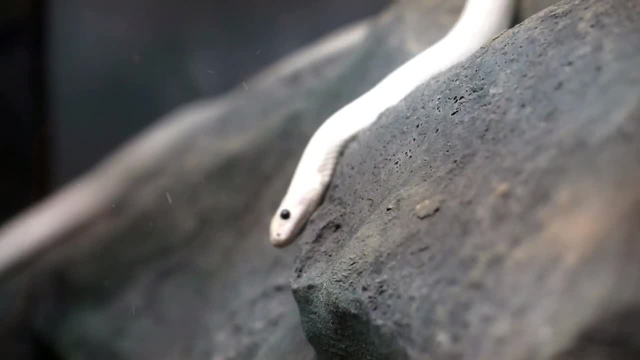 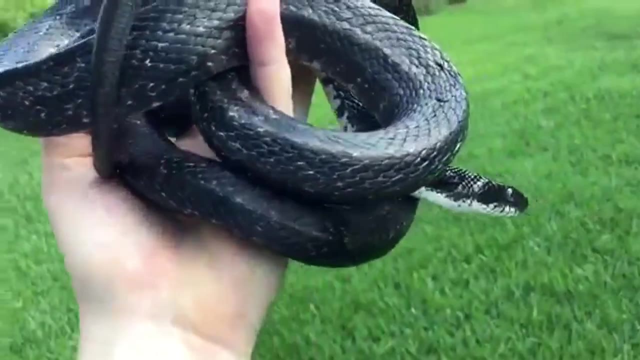 common in the United States. Its main prey consists of small mammals, lizards and other reptiles, including its own species, though they constrict and eat whatever they can. Contrary to popular belief, however, constrictor snakes don't crush their prey Rather. 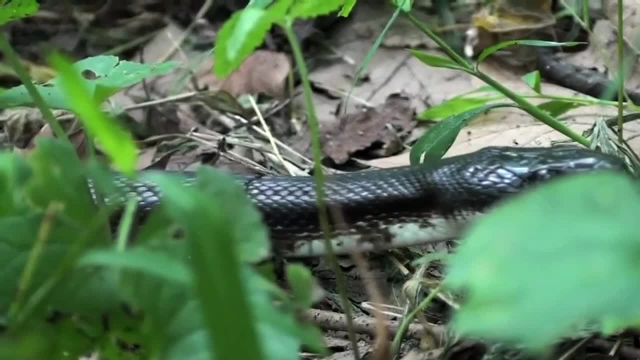 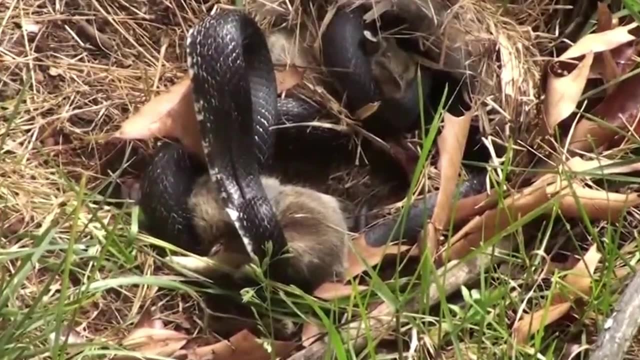 they suffocate them. Careful listeners to this flip, for instance, will notice a high-pitched squeaking noise at the start of the video. Unfortunately, that isn't the most visible baby- It is its siblings- calling for help from somewhere within the snake's encircled snare. 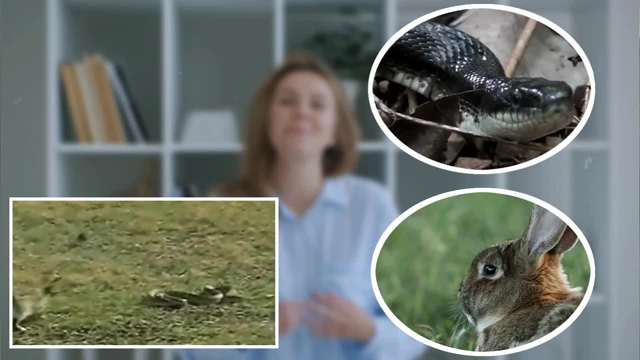 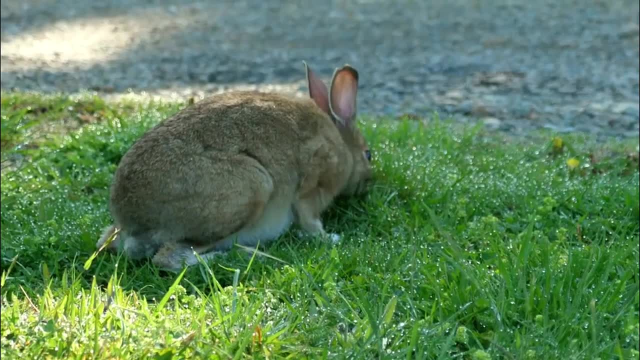 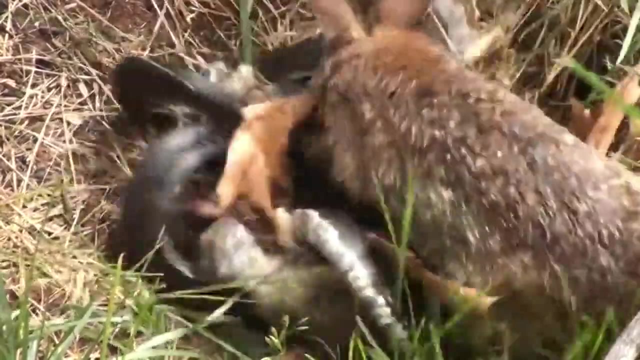 That was the remaining baby giving an alarm call, Dana Kremples, the biologist at Florida's University of Miami, said explained to National Geographic. Luckily, the call was answered by a very angry mother rabbit who dropped like vengeful lightning on the snake. The black rat snake instantly let go of the baby. 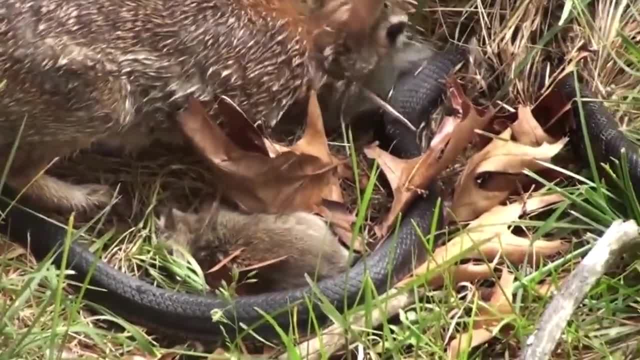 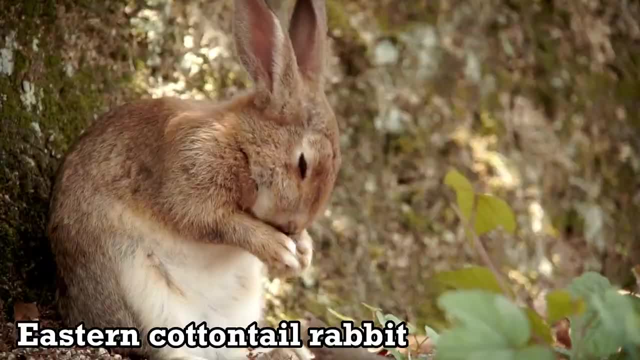 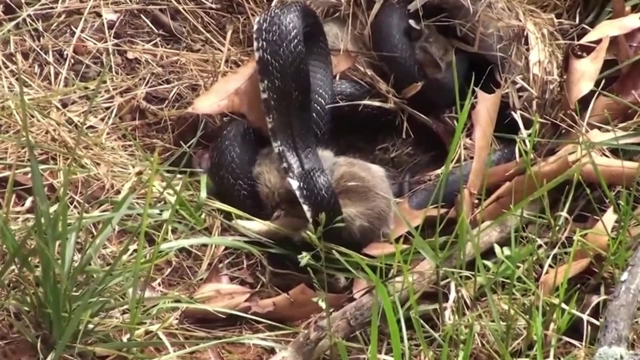 bunnies when angry mama pounced and a tiny fluffy form can be seen darting away from the unwrapped mass. Mama bunny, by the way, is an eastern cottontail rabbit. This species will fiercely defend its nests, As shown by Mother Dearest here, the cottontail checked on her baby's neck. 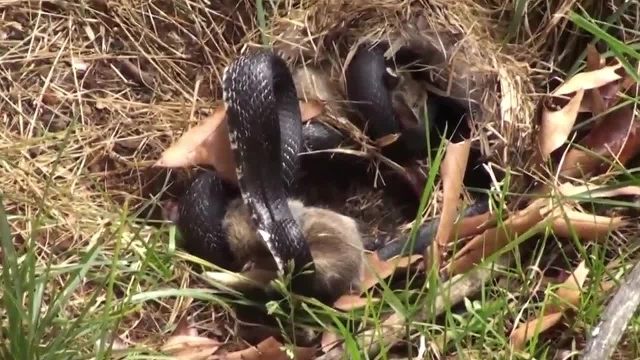 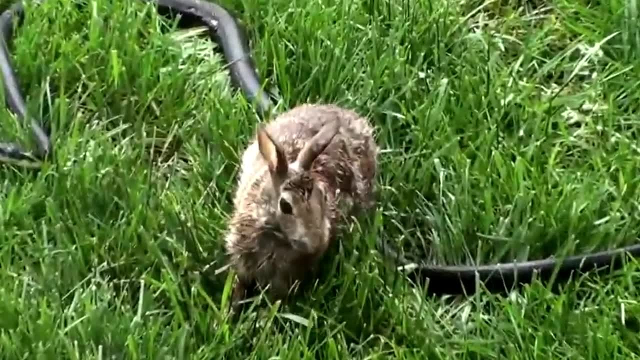 but the hungry rat snake had already squeezed the life out of two of them. Just as she realized that her children were dead, however, the serpent made the mistake of raising its head to strike and got a face full of enraged rabbits. The snake seemed surprised by the rabbit's ferocity. 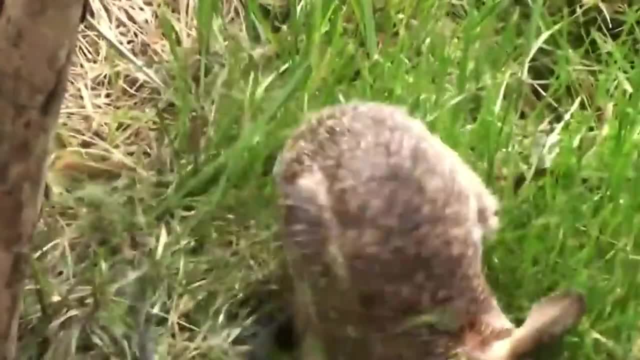 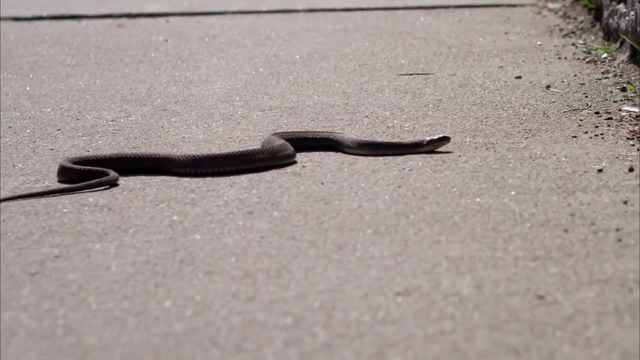 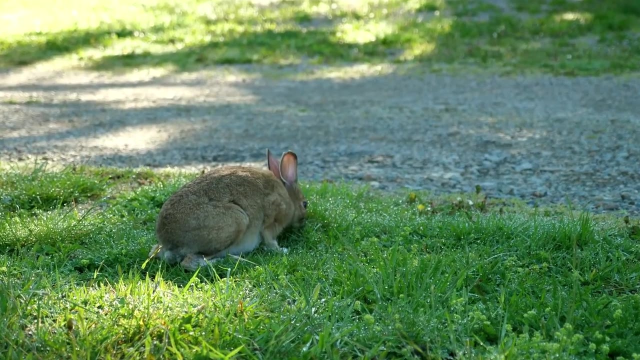 as the people recording it were Indeed. after a few attempts to defend itself against the darting back and fourth onslaught of mama cottontail, the snake made the sensible choice of escaping. But unexpectedly, the furry fury gave chase. Mother rabbits, after all, are a force of nature. 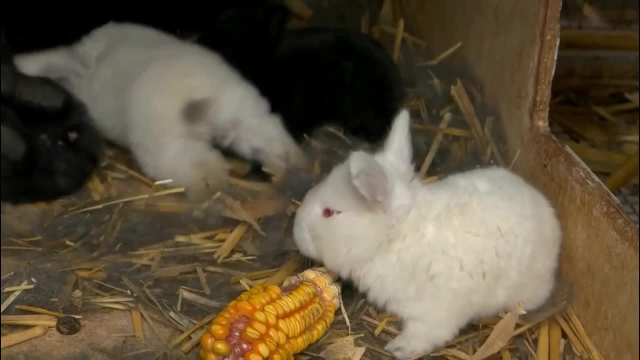 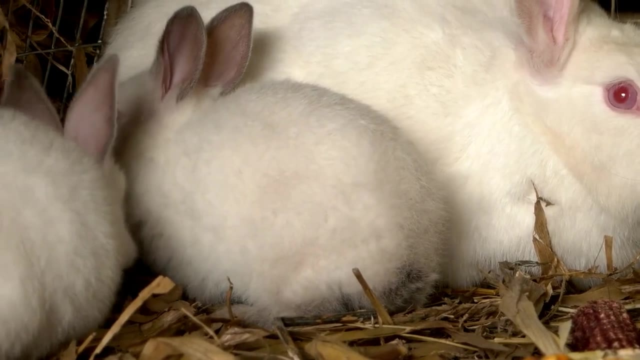 when it comes to defending their nests. Their bunny babies are born blind and helpless, and they have absentee fathers. The babies therefore rely on mommy for protection until they can defend themselves. Mind you, anyone who's seen Watership Down will know the 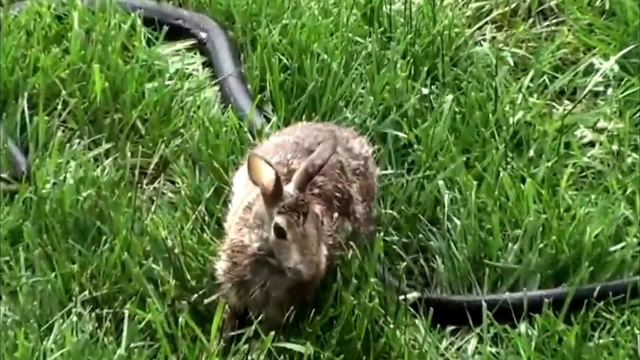 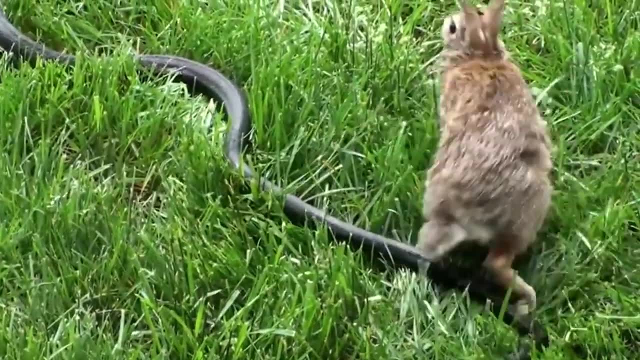 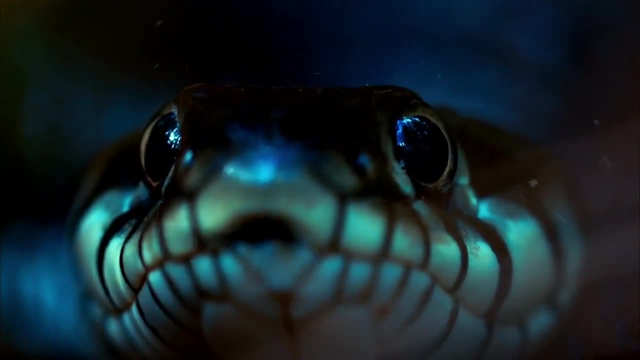 kind of brutality rabbits are capable of, And mother rabbits have a go-to move when it comes to predator disempowerment. Here, then, the rabbit pounced on her opponent and sank her teeth into it. She then flipped onto her back, turning the snake with her, With her sparring partner on top. 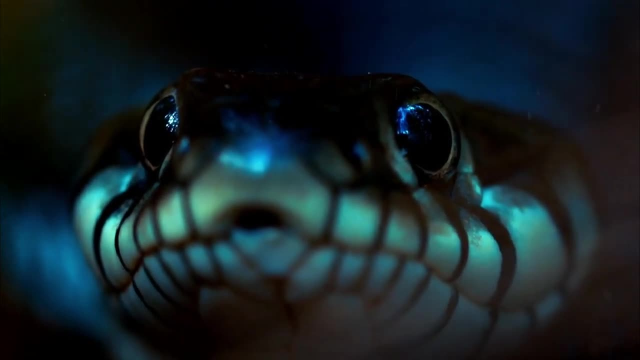 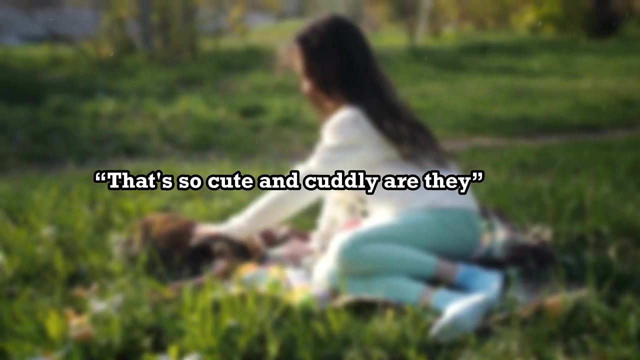 of her. the rabbit used her powerful leg muscles and sharp claws to take her enemy's stomach in an attempt to rip out his entrails. That's so cute and cuddly, are they? Crumple said Indeed, Elmer Fudge should be grateful that Bugs Bunny wasn't female. 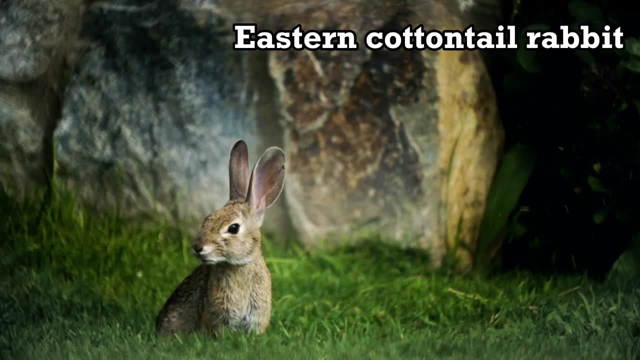 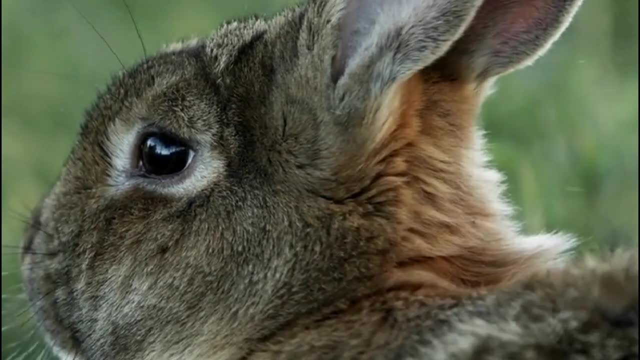 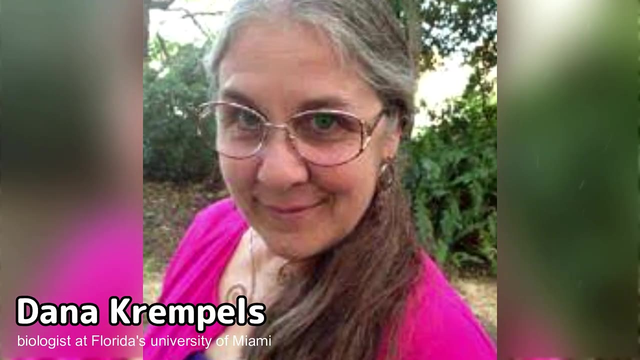 The Snake Attacked was allowed to happen because cottontails don't spend their daytimes in their nest or fear of drawing attention to their babies. Instead, they patrol nearby and come back periodically, when the sun rises and sets, to check on their little fluffers. Crumple's further told National. 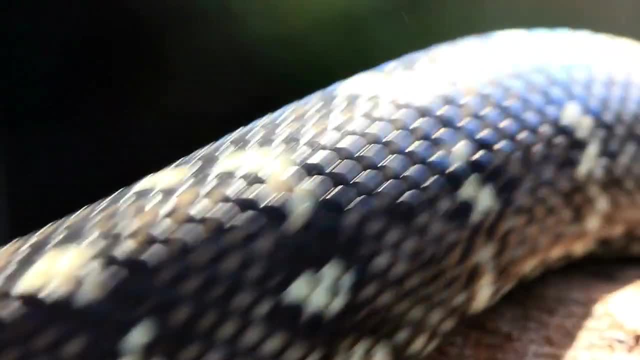 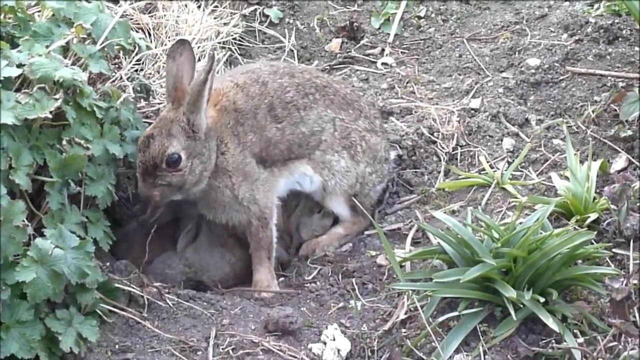 Geographic readers. But the cottontail's likely aim was to scare the snake or wounded badly enough so that it wouldn't come back, And from the desperate attempts the snake in the video was making to get away, it probably doesn't want to be. The snake was so scared that it tried to escape the rabbit's trap. However, it didn't be able to get away and the rabbit was still in the nest with its scythe. The snake was also in the nest with its scythe. The rabbit was not able to get away. The snake used its scythe to come out of the nest. 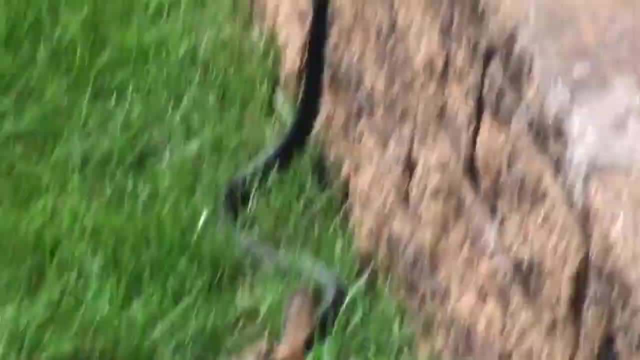 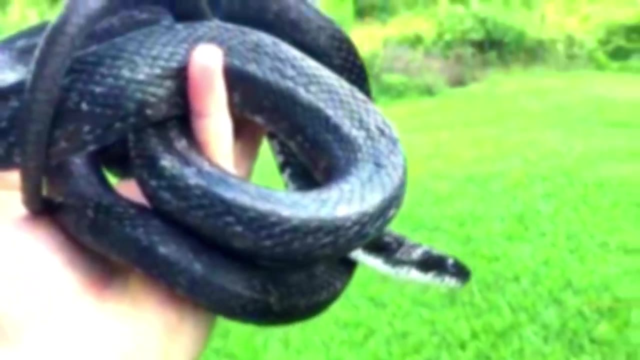 but it was unable to get away. Indeed, the snake even attempted to lift itself over a wall to escape the battling bunny. It stood a good chance at that. Black Rat Snakes are skilled climbers. They can even scale tree trunks with nothing but their coils to help them. 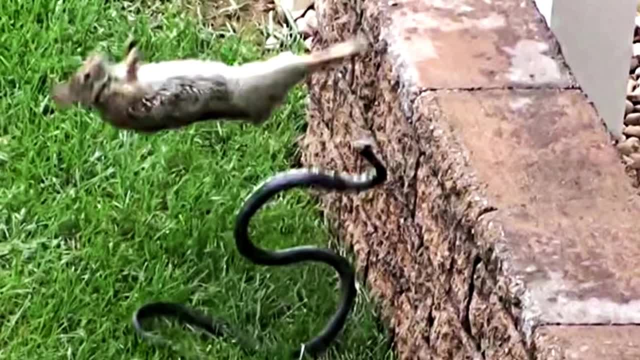 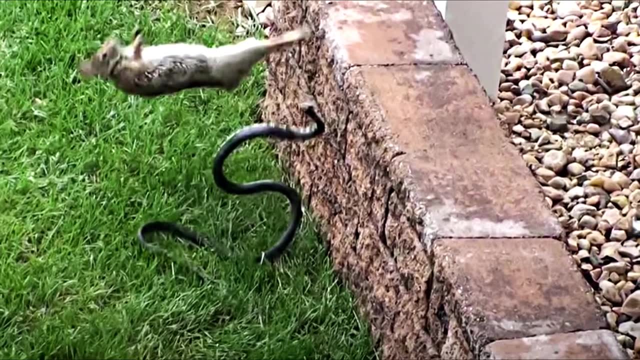 But the shaken serpent wasn't quick enough and Mama Cottontail caught up again, sinking her teeth into its tail. The bunny yanked the snake back into the metaphorical ring and into another rolling flurry of kicks. Black rat snakes can release a pungent musk to deter predators. 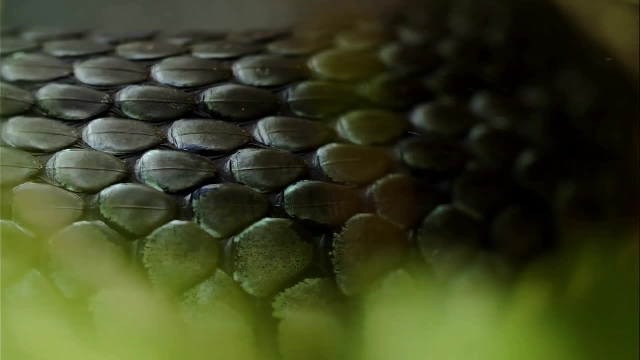 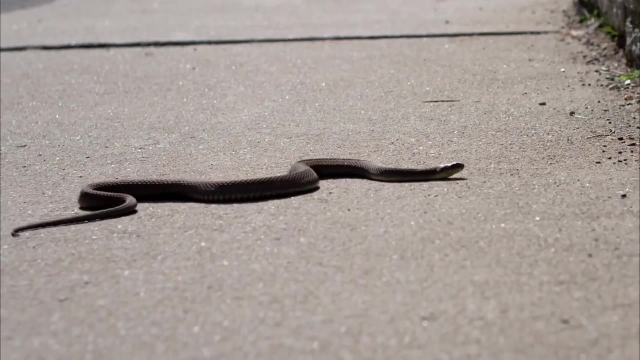 but if it tried that tactic already, it was clearly ineffective against the rampaging rabbit. In fact, even though the snake had tried to retaliate with some vicious bites, all it really seemed to do was bring its head closer to the furious mother cottontail. 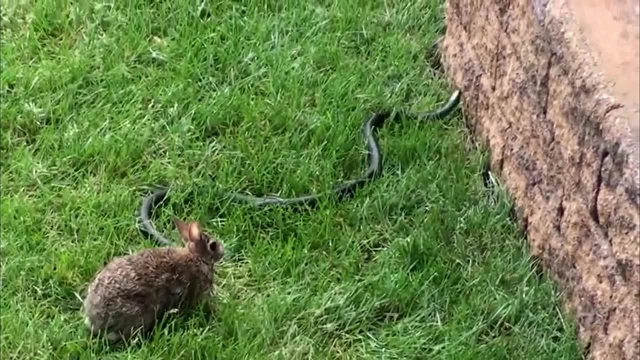 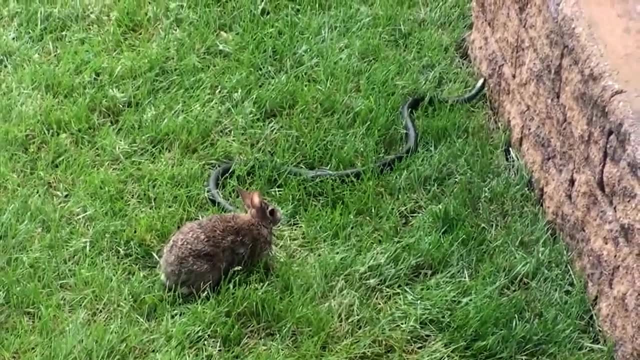 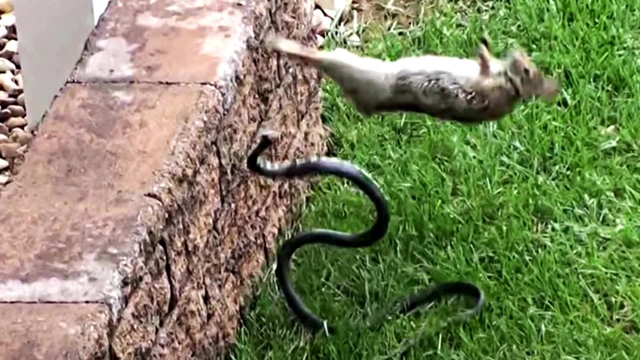 However, the exhausted-looking serpent finally made one last attempt to strike back and snapped its head toward the bunny. Unfortunately, it was the worst move that it could have made. The lightning-fast rabbit was simply too quick and leapt backwards into the air and kicked out with her hind legs. The amazing move looks like something straight out.